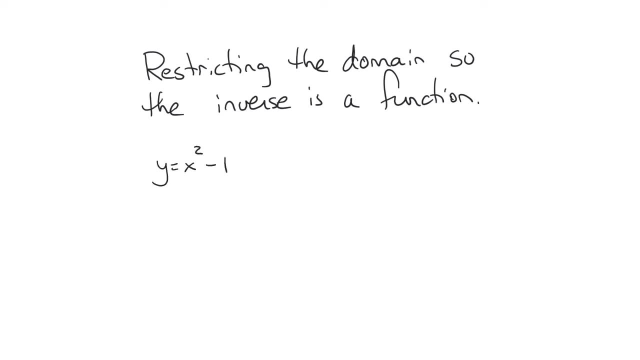 And the function that I want to use right now is going to be this function: x squared minus 1, y equals x squared minus 1.. So first of all, let's take a look at the graph And I want to focus our attention on the graph. okay, 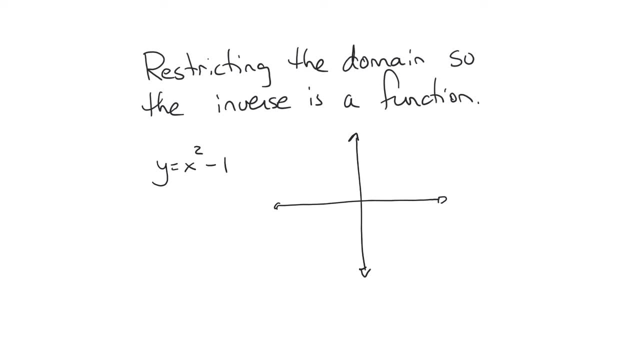 Because I want to get a visual sense of what's going on here. So I'm going to graph this: x squared minus 1. And really it's just a parabola that's been shifted down one unit here. okay, It's going to look something like that: 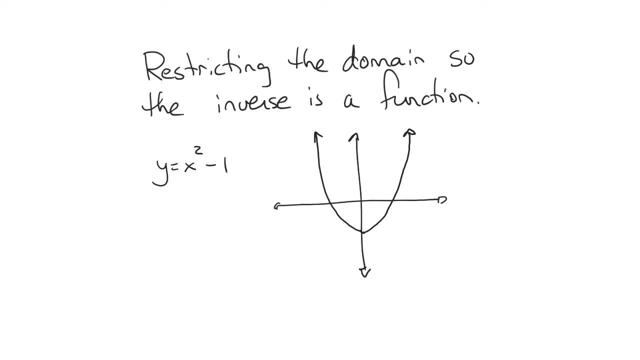 Now I'm going to find the inverse, And we do that by swapping the x and the y. Bring the 1 over equals y squared, and then I'm going to take the square root. And when I take the square root, something special happens. 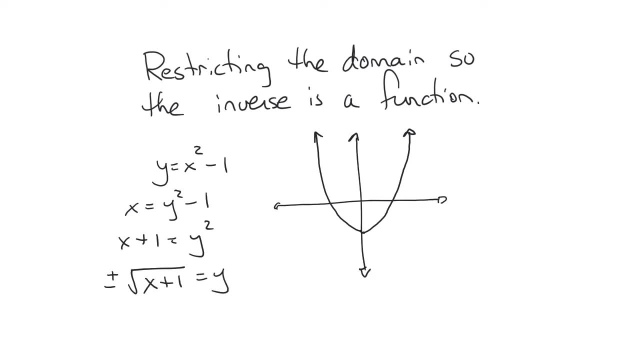 I get this Plus or minus square root of x plus 1.. Now I want to illustrate what's going on here. So what I'm going to do is I'm going to take the parabola that I've got here and I'm going to color the left-hand side red. 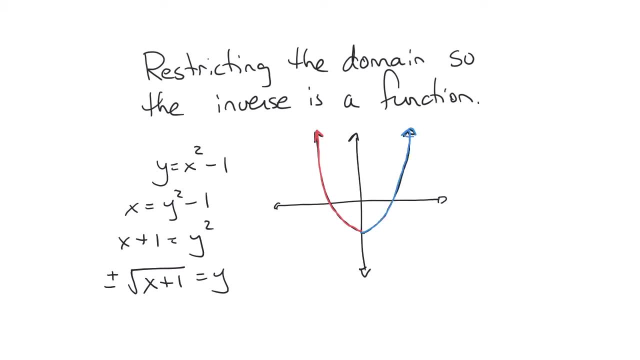 and we're going to color the right-hand side blue. Now, when you found the inverse here, your inverse is automatically broken up into two parts: The positive square root of x plus 1 and the negative square root of x plus 1.. 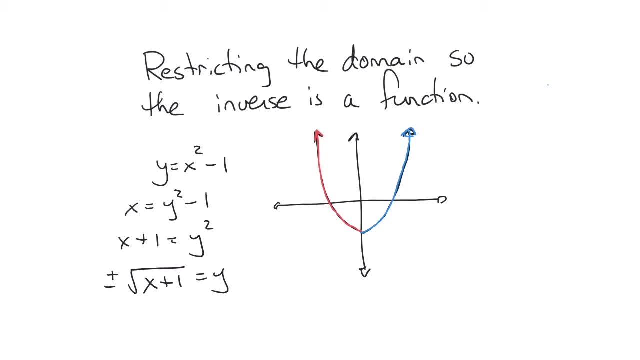 The positive square Root of x plus 1,, when I plot it here, is going to look like this: It's going to start at negative 1, and it's going to go up like that: The negative square root of x plus 1 is going to start here at negative 1,. 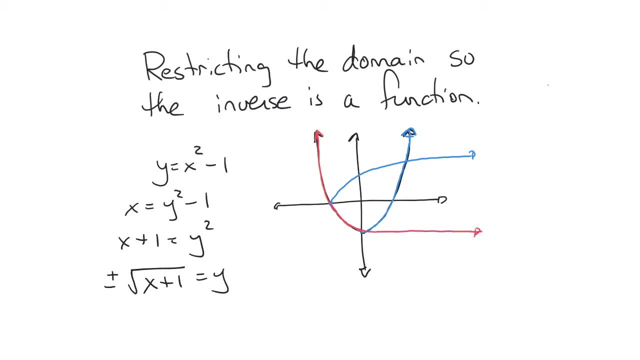 and it's going to swoop down. Now my diagram isn't really doing justice to that. That probably should have swooped out a little bit more like that and then come around. Anyway, you get the idea, You get the idea. 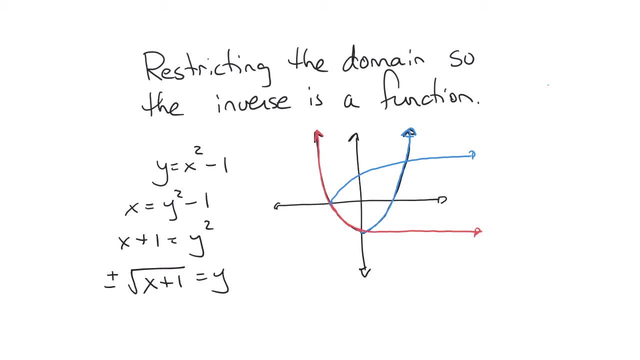 I'm just going to undo that last little bit there, But you get the idea, okay. So this right here is my positive, The red here is my negative. Now, clearly, when I draw a vertical line through this, oops, when I draw a vertical line through that inverse, that is not a function. 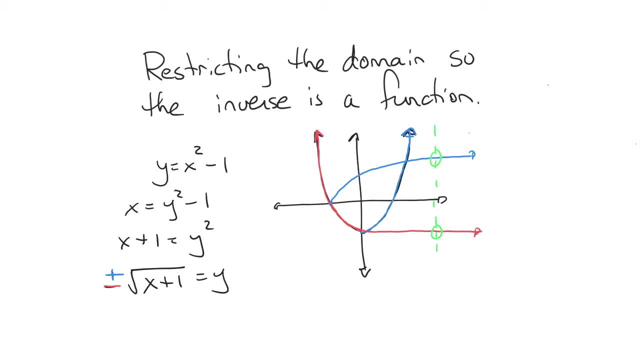 That inverse is not a function, because my vertical line hits it more than once. So what I want to do is I want to restrict the domain on this so that when I find the inverse, the inverse is a function here. Now that's going to take just a little bit of thinking here. 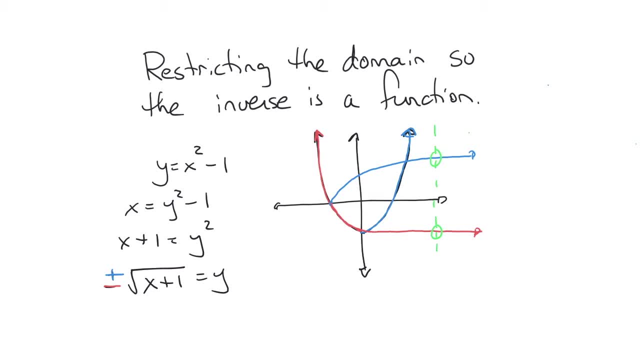 So let's take a look at this again And what We'll force a restriction to happen here. okay, Whoops. Now I'm trying to move to the other screen here. It's not letting me do that, So let me do this. 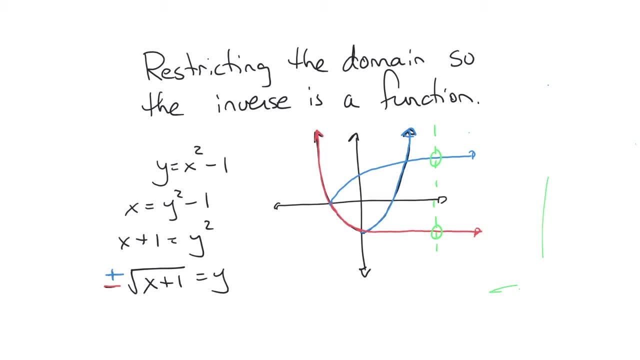 We're going to erase what we've got here. Now I'm going to start this again here. Whoops, It's not letting me do it. Here we go, Okay, So let's try this again, And I want you to see what's going on here. 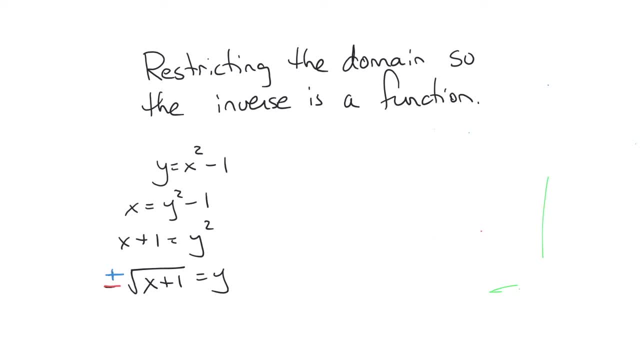 Sorry, This particular Program isn't doing exactly what I thought it would do, And that's okay. So now let's draw that, that grid again. So here's my, here's my parabola. Now, what I'm going to do is I'm going to restrict the domain. 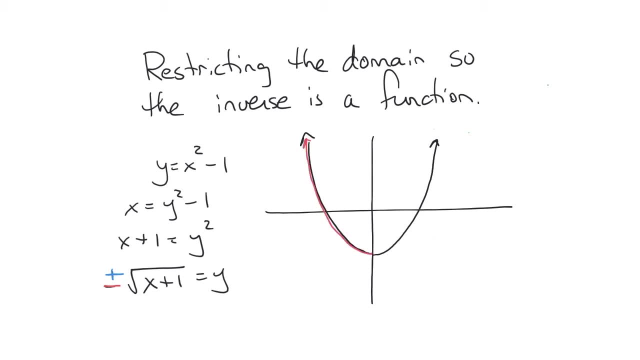 I'm going to pick a point here and I'm going to, I'm going to draw this on here again. There's my red, there's my blue. I'm going to pick a point. Let's pick it right here, Okay, so this is my A. 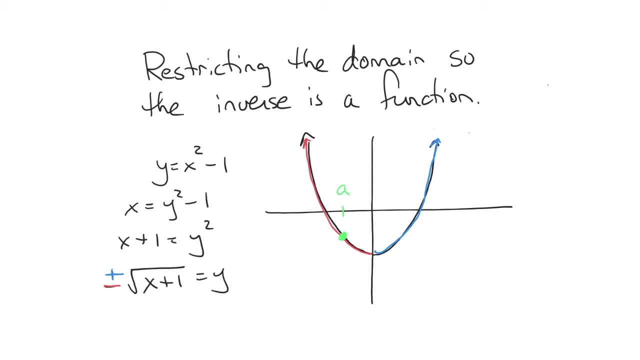 I can pick any point I want along the function here in the domain of the function, any X value I want. But when I do that breaks this into basically two intervals that I'm interested in: the values of the parabola to the left of A. the values of the parabola to the right of A. 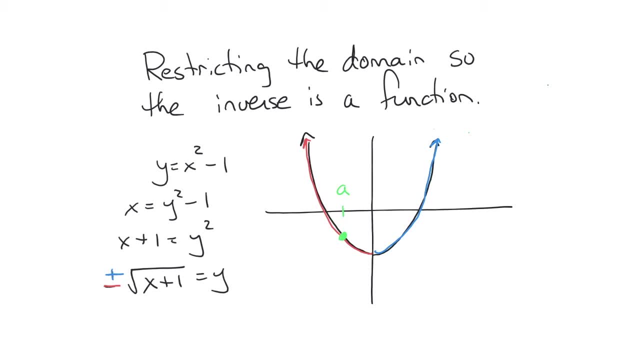 So what we're going to do to start off with here is: I'm going to restrict my domain. I'm going to look at values along the domain here that are, strictly speaking, greater than or equal to A. So I'm going to look at just. 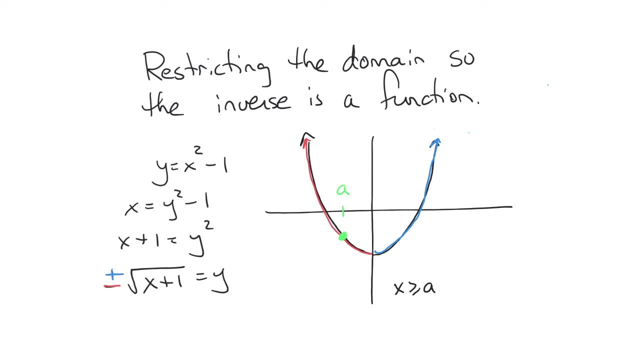 Just where X is greater than or equal to A. Now, what that means is: I'm looking at this part of the graph here- Okay, I'm going to get rid of that portion right there, And so I'm just looking at this portion of the graph. 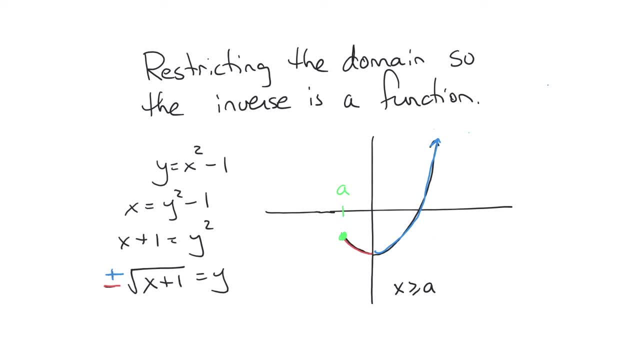 Now, when I find the inverse, what happens here is: I've got this, this blue part here. It starts at negative one. The blue part still swoops out like that, But my red portion only goes out so far. It Only swings out to basically where, where that A value, where that inverse would be down here. 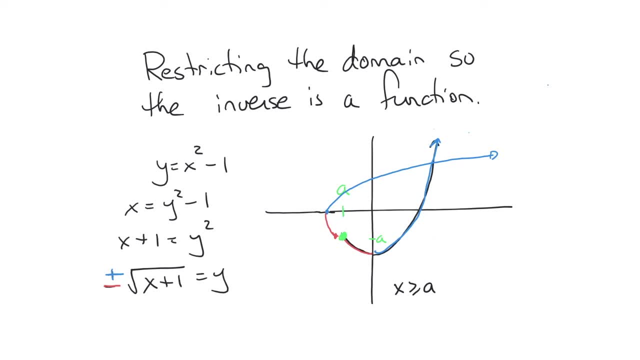 This would be like where my A is, because I'm flopping them here, So I've got that little portion here. Now that isn't a function, Because I've got both the blue and the red portion, When, whenever I find the inverse, the blue is always going to be over top of the red. 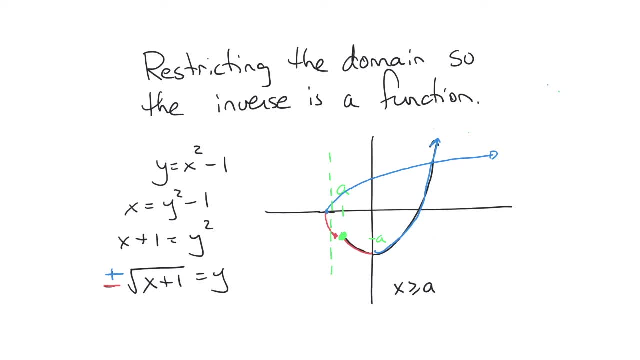 The red portion will always be below a portion of the blue, So, as a result, I'll always be able to Draw a vertical line through that. Now, if I go back, we clean this up here a little bit here. Now I'm going to have to be a little careful here because I don't want to have to redo everything. 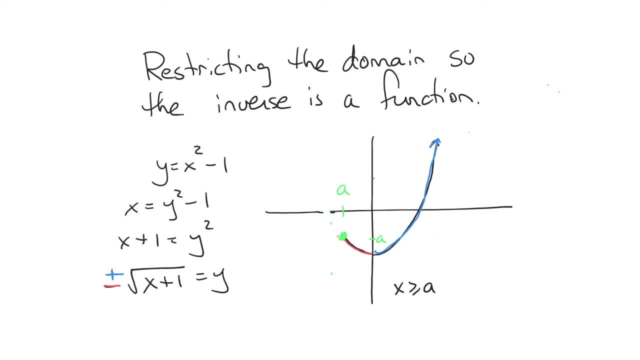 I can change what it is that I that I take here. So I had this, this original function here. If I take now and restrict my domain, not so X is greater than or equal to a, but so that X is, let's say, less than or equal to a. 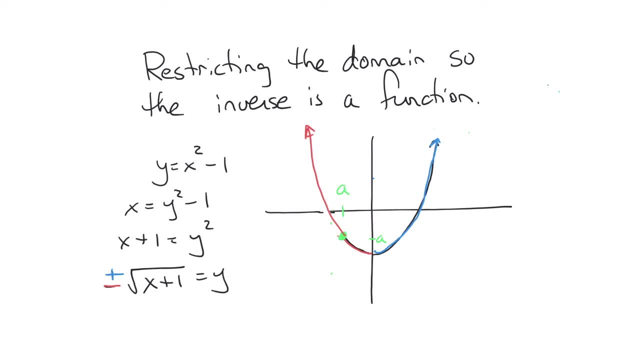 Okay, let's say that X is less than or equal to a, then what happens here is: I'm getting rid of this portion of the graph. Okay, I'm going to draw in those remaining little bits there, just so that I clean that up here. 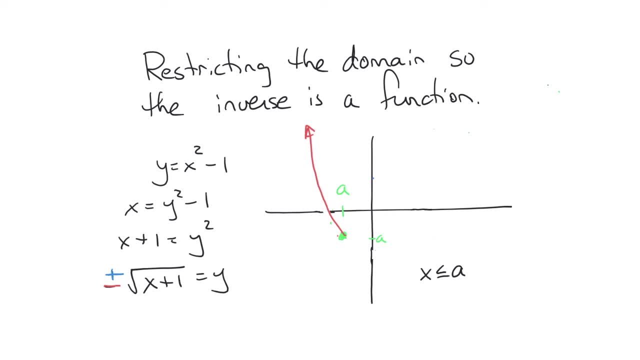 Now, if I find the inverse of that, well, there is no. there is no blue portion of this graph, It's only a section of the red portion that was underneath. I'm going to start at that. The inverse of that point, a comma, whatever the Y value is. 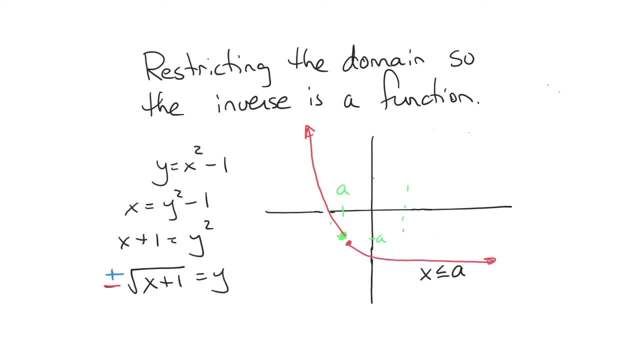 And when I invert, it's going to come down like this: This particular portion Is a function. no matter where I put when, no matter where I put a vertical line along this portion of the graph, it is going to be a function. So what happened there? if you think about it, I chose a point along the graph that was to the left of the vertex. 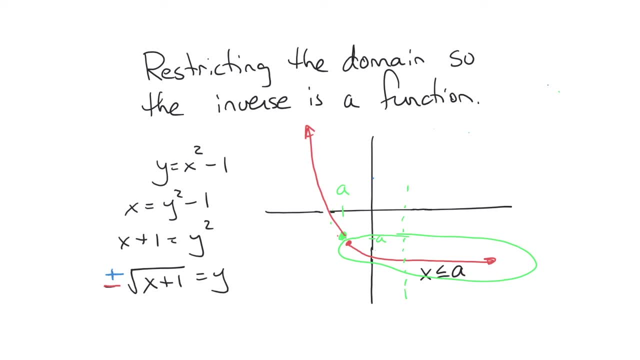 So when I, When I did my restriction on the domain, I had to carry on from that point and keep going to the left. Now let's take a look at another way. This could work here. Sorry, it's taking a little bit of time here. 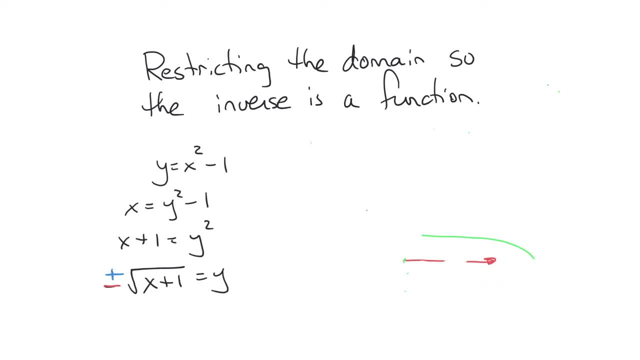 This should have allowed me to go to another screen, but for some reason, as soon as I got into recording, it decided it didn't want me to do that. So now, if we take a look Again, here's our, our parabola. 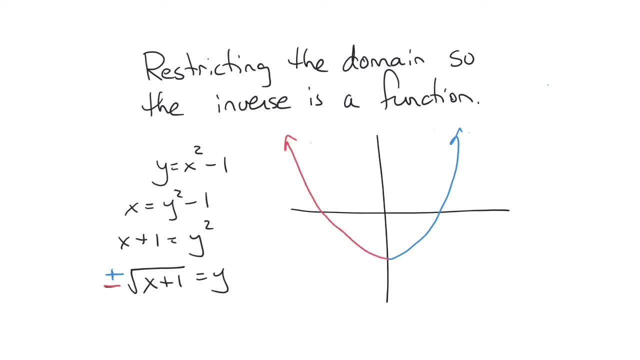 We're going to go blue up here, We're going to go red this way here. If I now cut it, let's say here: And we're going to make this my a. So I chose it again. I just choosing a point along the parabola. 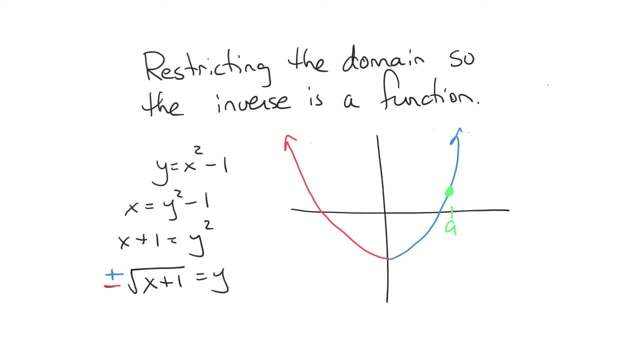 I can restrict the domain to either be to the left of a or to the right of a. Now, last time I chose it, Okay, I went to the left of a and that worked, So let's try that again. So now I'm going to get rid of the part of the graph. 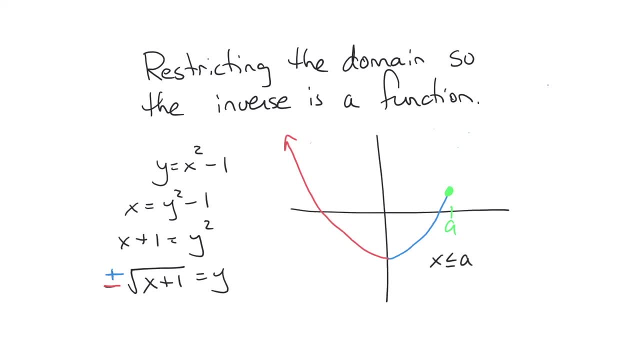 That's to the right, That's to the right of it. So all I'm going to look at is this right here, When I find the inverse of that, it's going to start here at that, where that negative one is along the x-axis. 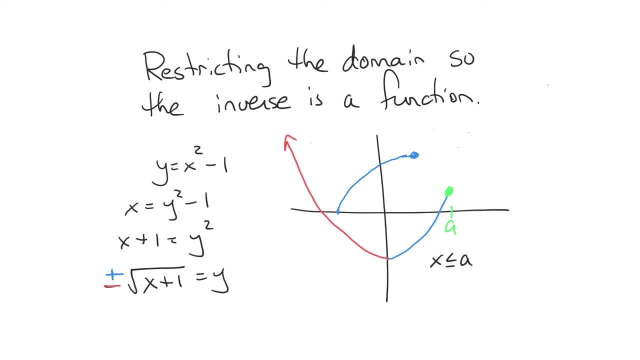 There's my blue, and my blue is going to stop right there, Okay, at the, at the inverse point of that end point there, And then my red is going to come along, kind of like that, And away we go. Now, that is not a function. 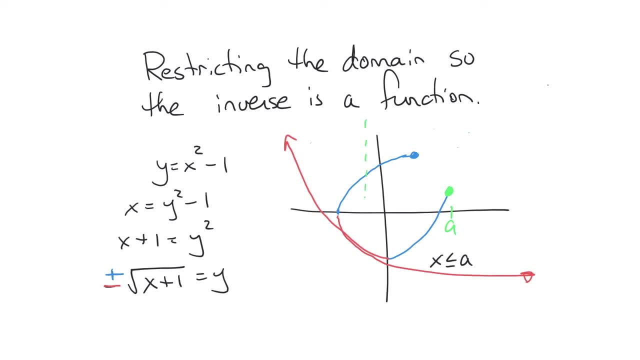 Okay, because I've got this section right here where I've got the blue part that I inverted Over the red part that I inverted right there and right there That's not a function, So that didn't work. So let's, let's take a quick look at this again here. 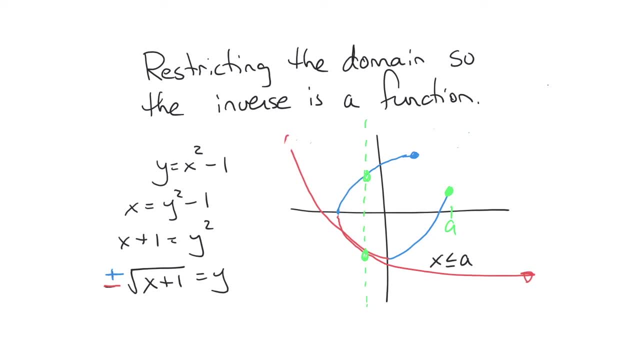 Well, what? what should we have done? Okay, we'll clean this. We'll clean this right up here. Gonna start this from scratch. Okay, Cleaning it up, There we go. So now we'll draw Our parabola one more time. 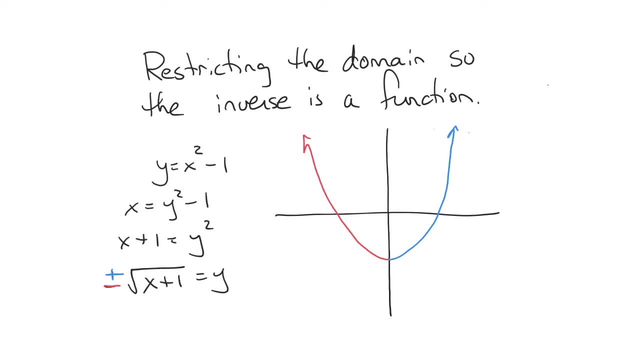 We're going to go up here like this. Then here's the red portion. I'm going to pick this point right here. There's my a, but this time I'm going to restrict my domain, So the domain is greater than or equal to a. 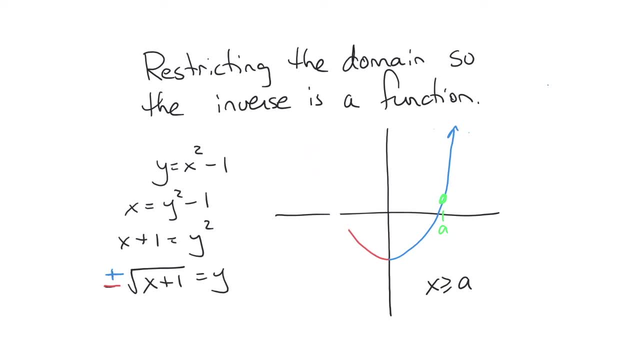 That eliminates for me this portion of the graph up until a. So now, when I find the inverse- Inverse of that, notice, there's no red part. Basically, I'm going to find the inverse point of that, a comma, whatever the y coordinate is. 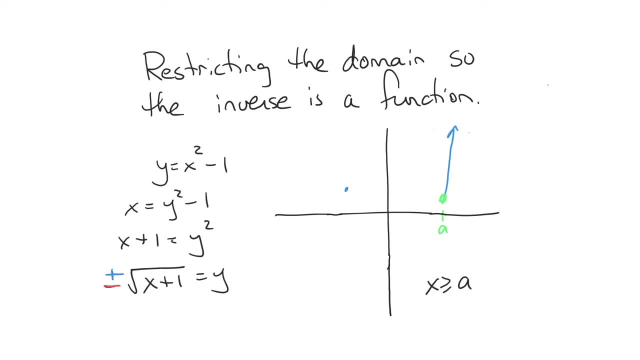 It's going to go over here and that's going to- or sorry, No, not over there, It's going to be somewhere over here, really- and then it's going to swoop up like that and that function there. So that is going to be a function, and it's because I'm restricting. 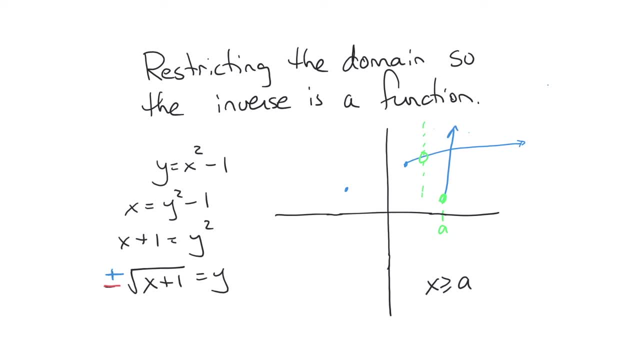 the domain in a way that doesn't. that doesn't allow me to have both A red portion and a blue portion, because anytime I invert that parabola here, the blue portion is going to be over the red portion, and I don't want that. 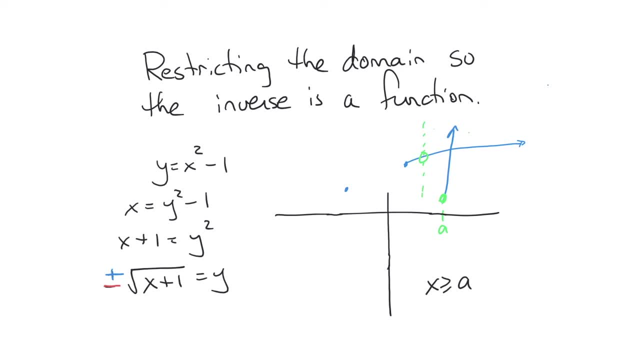 So if we can kind of summarize what's going on here, let me. let me redraw the parabola again, going right, right back to the beginning. Okay, Here's, here's the blue portion that goes over here. Here's the red portion. 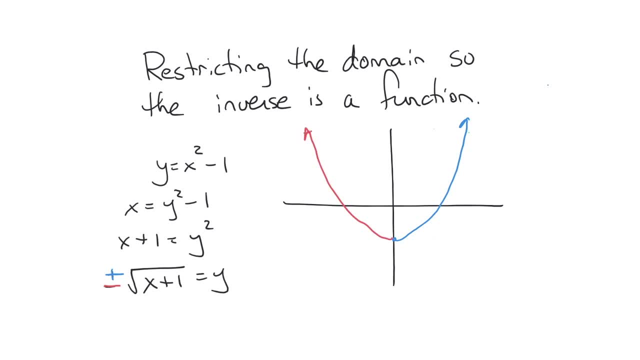 That goes over here. So now here's my vertex. Okay, I've got the vertex here at the point zero, comma, negative one If I choose A. Okay, Well, that's sorry, That was horrible, I got to rewrite that. 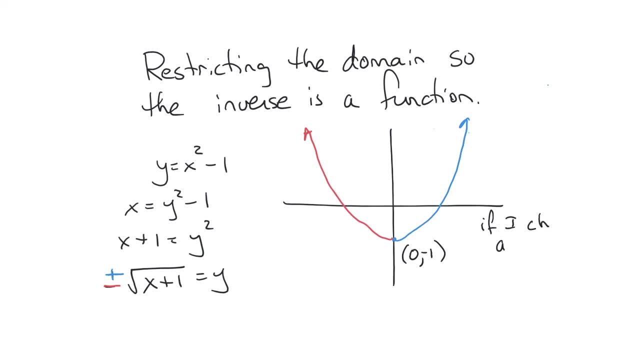 That's embarrassing. If I choose A less than zero, or let's say less than or equal to zero, Then my Domain Is X less than or equal to a- Whoops. But If a is greater than or equal to zero. 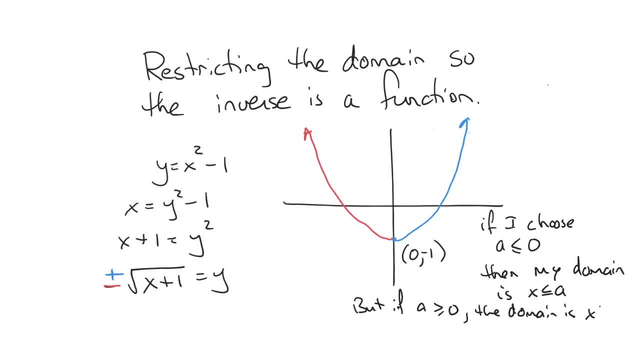 The domain Is X, greater than or equal to a. So let's just take a look at it again. If I choose, if I choose a point out here, And here's my a, I want to restrict my domain To the points left of that point. 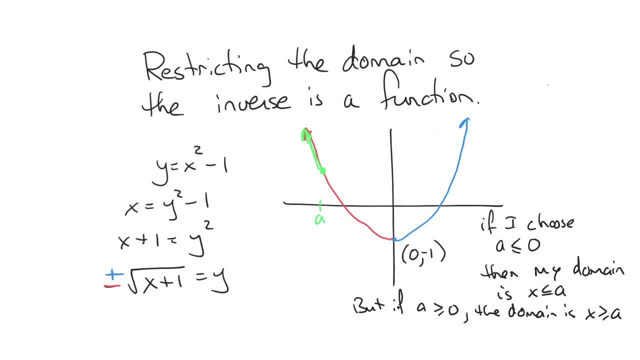 Because if I choose the domain to the right, it's going to ensure it's going to include both a red and blue portion And when I invert that those will be over top of each other. But if you chose, choose an a over here, then my domain has to be to the right of that point so that I don't include both that red and the blue portion.